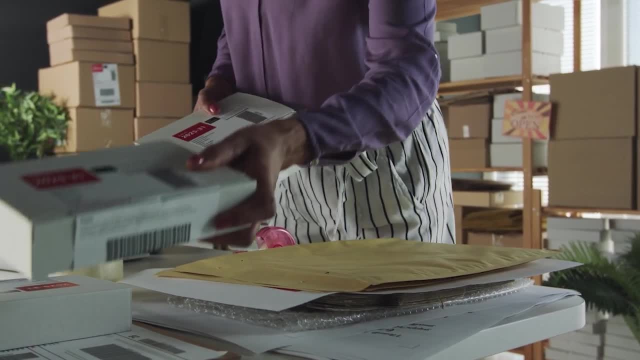 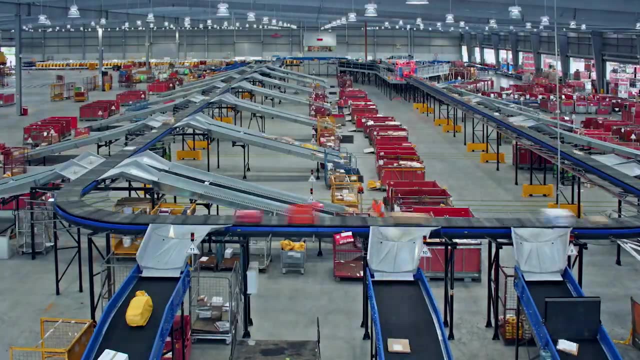 Humans are great at making classifications. We do this daily based on available observations and past experiences. But what if we need to make classifications on complex systems or make them thousands of times a second? And of course, we want them to be reliably accurate. 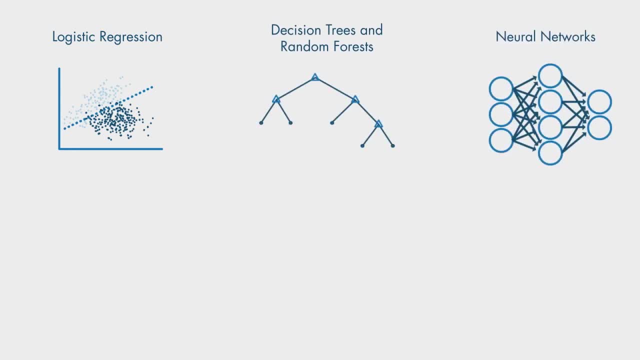 Well, we can use machine learning algorithms that give computers the ability to learn from data and make decisions. There are many different models. We'll look at a popular technique known as support vector machines or SVM. SVM are supervised binary classifiers. This means: 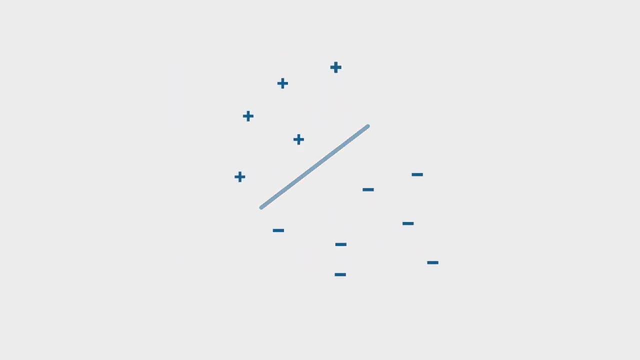 they use labeled data to learn how to sort observations into two classes. During the training process, the SVM learns how to best separate the data. It does this by finding a boundary that maximizes the margin between two classes. In this two-dimensional case, the 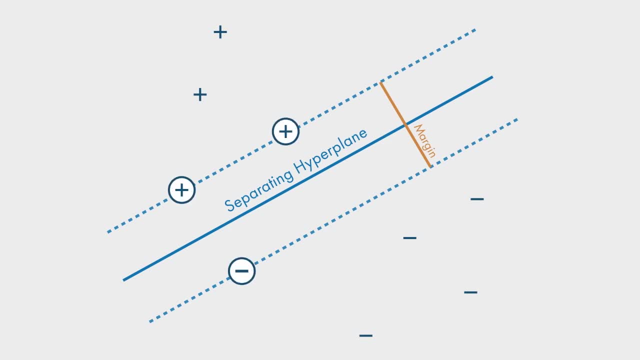 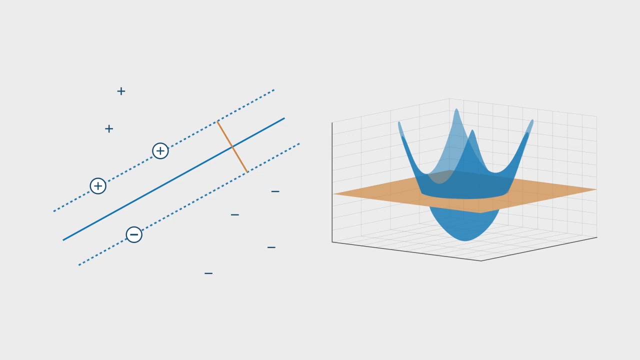 boundary is just a line. The data points that define the boundary are known as support vectors, hence support vector machines. You can imagine expanding this into higher dimensions as we add more parameters to our model. In three dimensions, the boundary between classes is a plane, and beyond that it's a 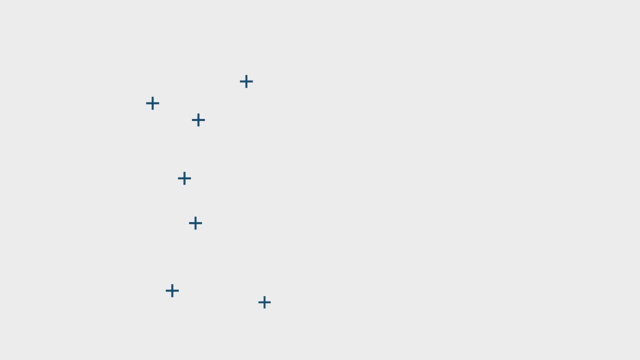 hyperplane. Most real data won't be linearly separable. How would an SVM handle a dataset that looked like this? There is no linear relationship to separate this data. SVMs can transform our data to higher dimensions to find an optimal separating hyperplane. 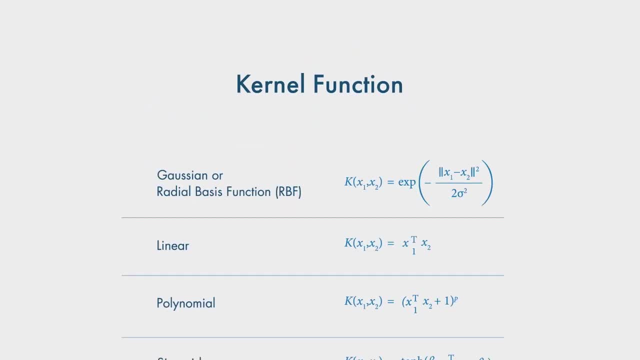 This transformation is called a kernel function. There are many types of kernel functions to systematically find the best transformations for our data. It's obvious that a circle can be drawn to separate the data, so we'll use the equation of a circle as our kernel function. 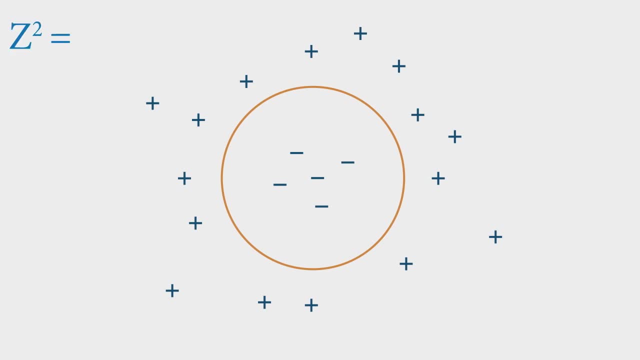 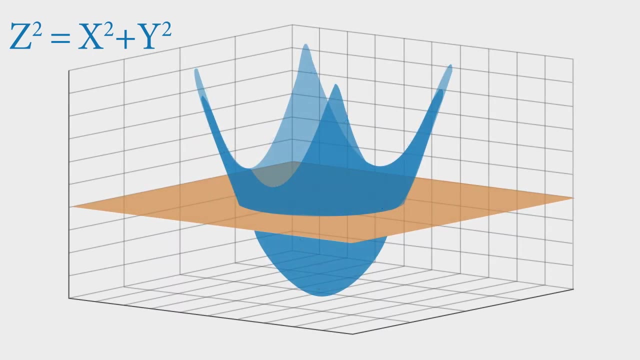 With the data centered around the origin. z squared equals x squared plus y squared. transforms the data into three dimensions so we can separate the two classes. SVMs are popular and widely used to solve classification problems. SVMs are also used to solve classification problems. SVMs are also. 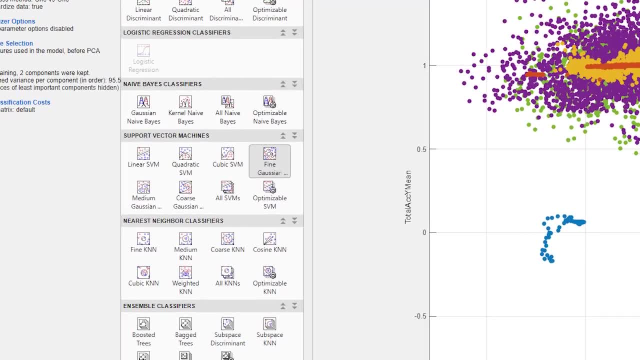 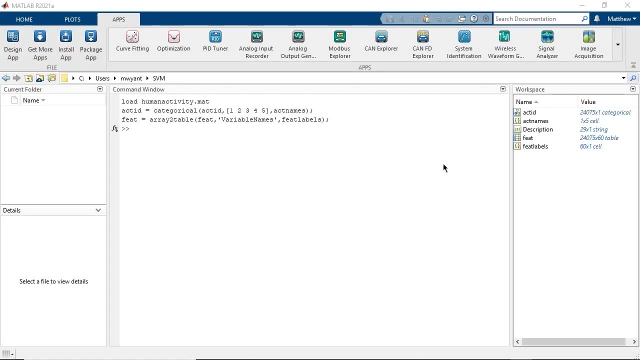 available alongside all other popular machine learning algorithms in the Classification Learner and Regression Learner app in MATLAB. Let's walk through a practical example using SVMs in MATLAB. First we'll load an example dataset built into MATLAB. This dataset classifies human.